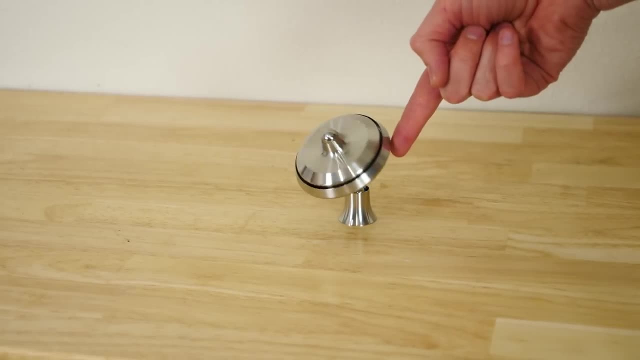 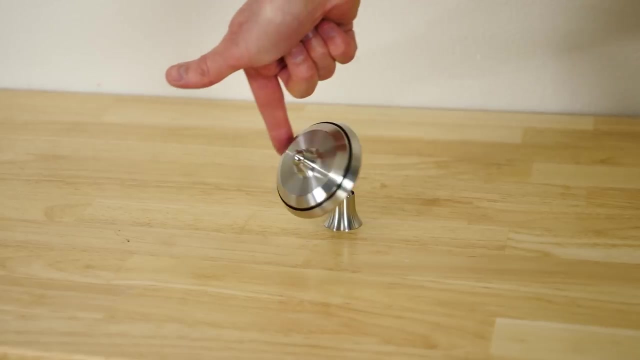 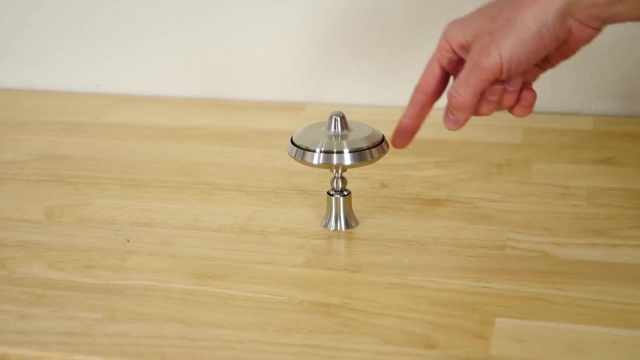 So if I try to slow its precession it drops, But if I try to speed up its precession it raises. So the ability to precess is what keeps it from tipping over. Even when it's pretty stable, it's still precessing a little bit. 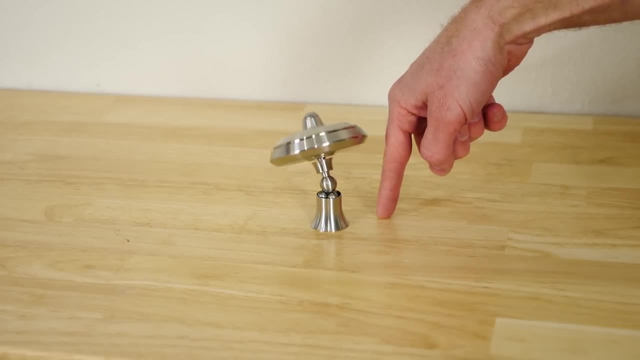 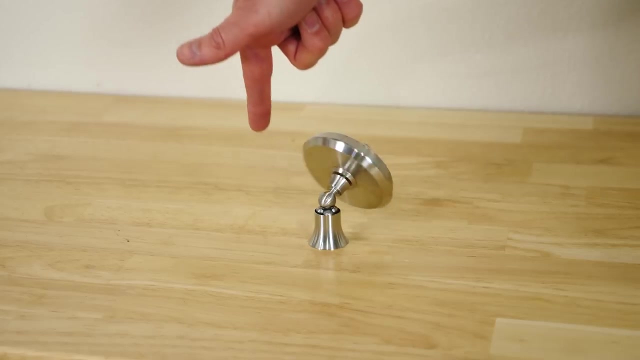 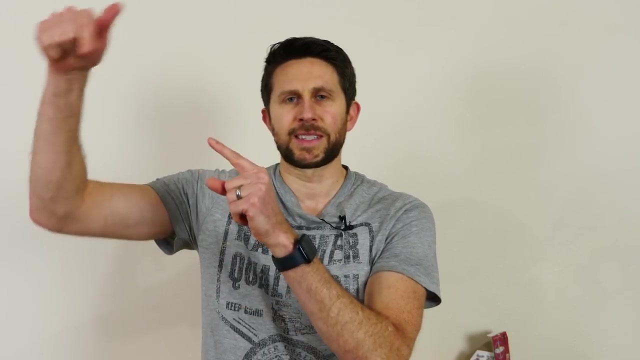 And if I don't let it wiggle like that, it wants to fall over. But then give it a little push with its precession And it comes back up. So the reason a gyroscope initially precesses is due to the force of gravity pushing down on it. 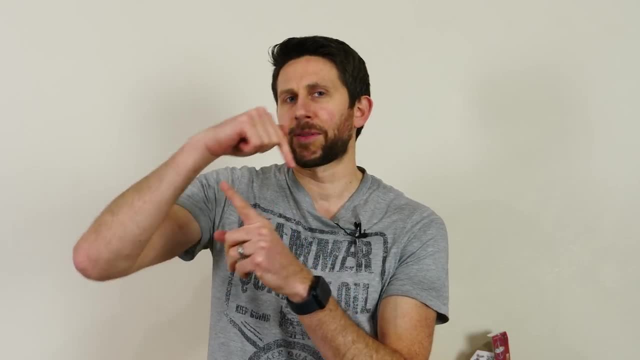 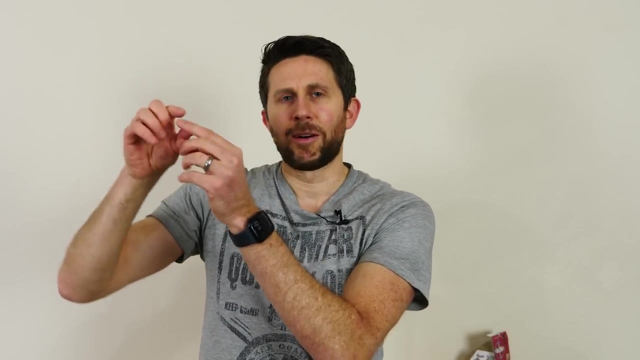 And due to the angle of torque on it it causes it to continually precess around in a circle, not getting lower or higher. But when it starts to precess around in a circle there's always some friction at the base there. 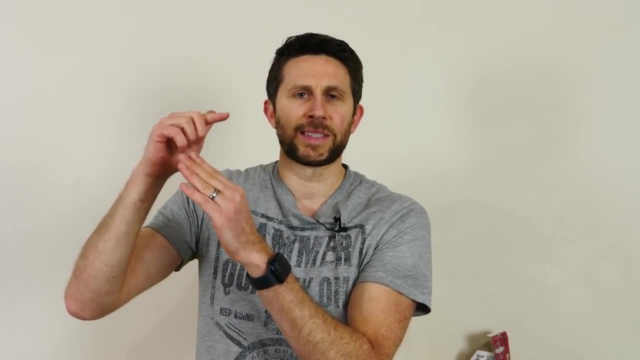 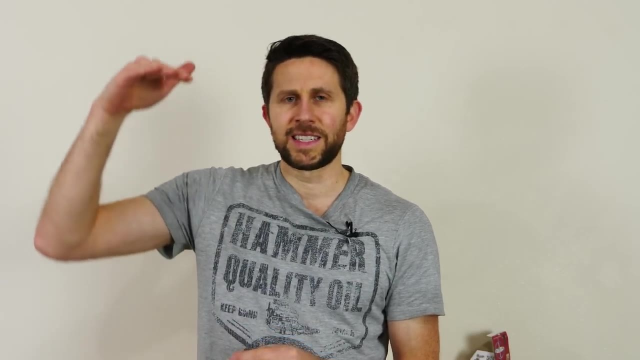 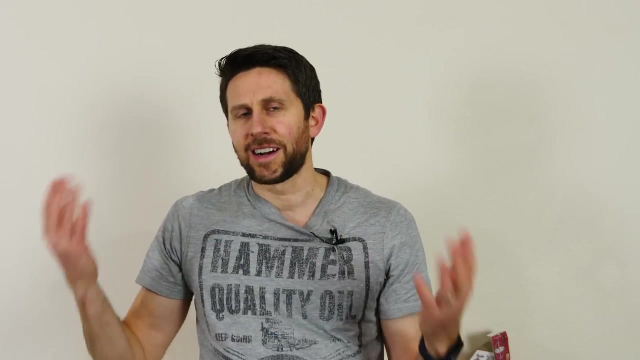 And so the base is applying some friction to it which resists the precession. And you saw that whenever we resist the precession, it causes it to drop even lower. So the more you resist it, the lower the precession. So the only thing that causes the gyroscope to eventually tip over is the friction on the base, not gravity. 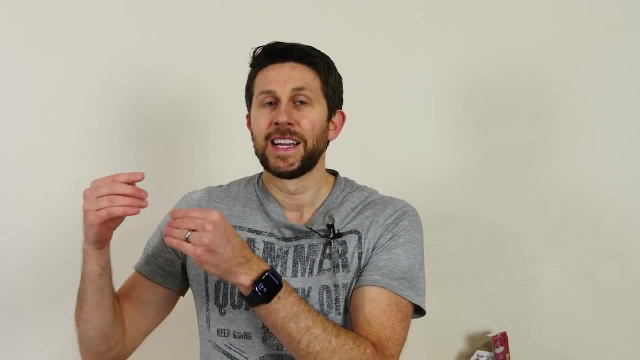 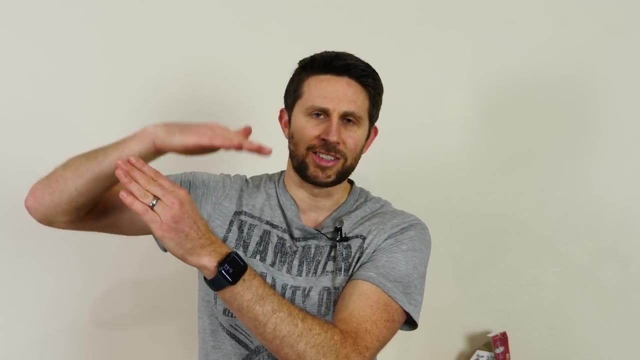 Gravity is what causes it to precess in a circle and that does cause the friction. But the friction is what causes the precession rate to slow down, get resisted and that causes it to drop down even lower. If you can reduce the friction of the precession, then you have another friction that starts to take an effect. 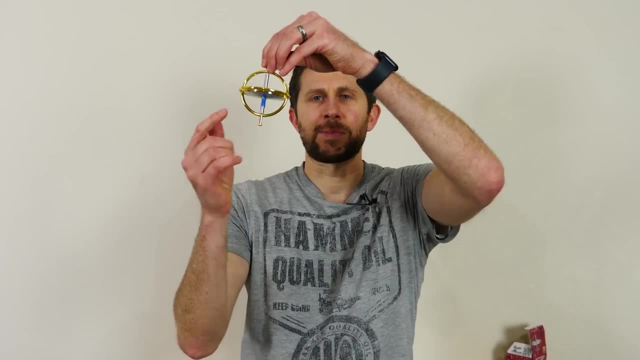 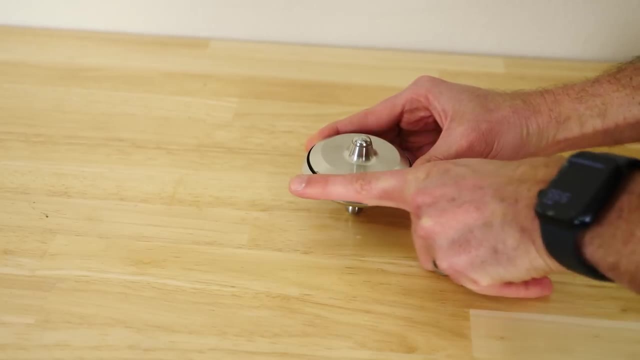 And that friction is the friction of the actual spinning gyroscope, So the friction of this axis here. So, on the spinning gyroscope, when you apply a force in the opposite direction of the spin, it actually causes it to precess the opposite direction. 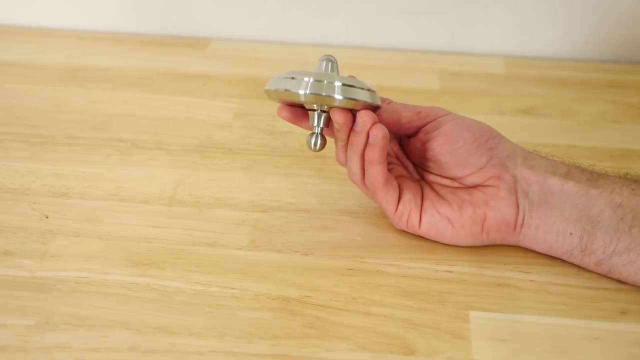 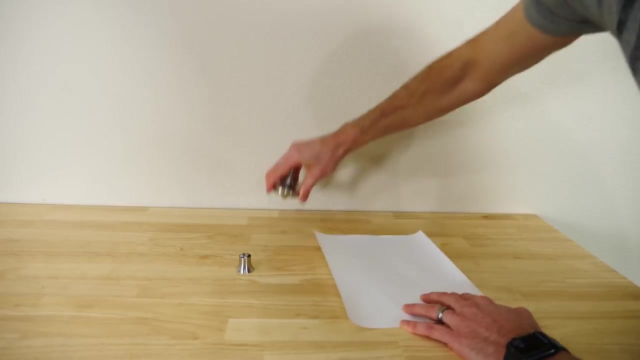 So it causes the opposite effect of the friction due to precession. So the friction around the spinning axis causes the gyroscope to want to lift up. So watch this. I have a gyroscope with a very frictionless base that just spins on ball bearings. 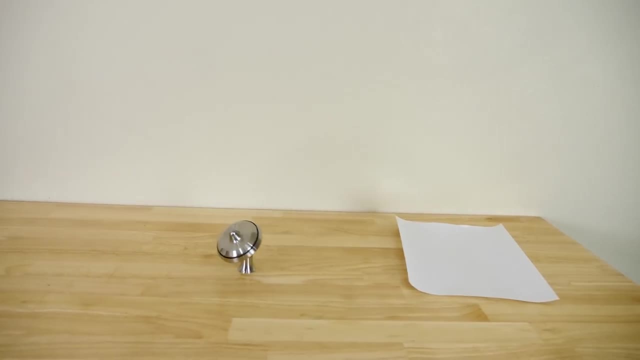 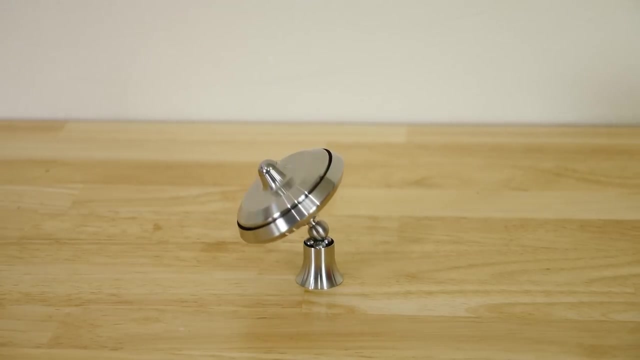 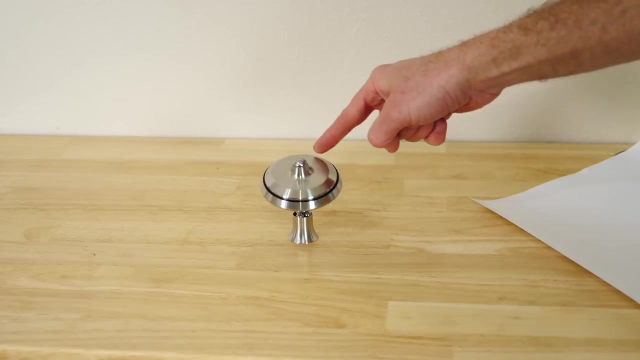 So it immediately starts precessing. But now watch what happens, So it gets completely upright again. So how can I actually prove that it's the friction, resisting the turning, that's causing the spin? Well, if I try to just give it some resistance like this, I'm actually stopping the precession as well. 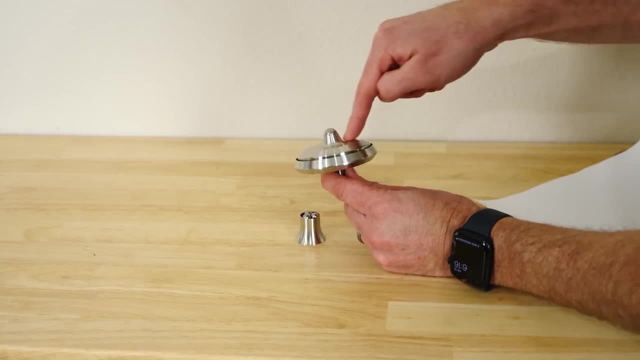 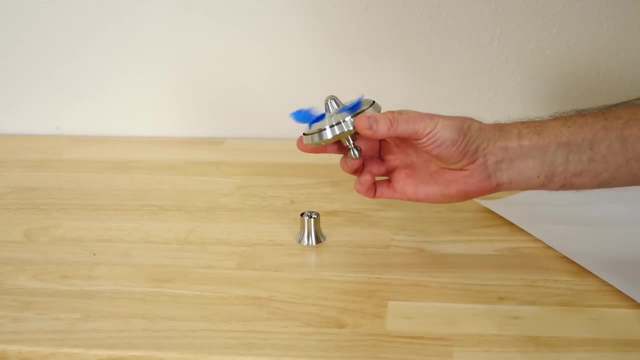 So it's going to tip over. So I have to find a way to only slow down the spinning without stopping the precession, And the way I'm going to do that is just to put some tape on the gyroscope and get it spinning. 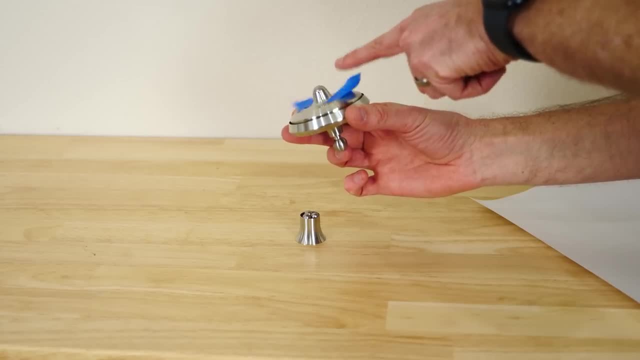 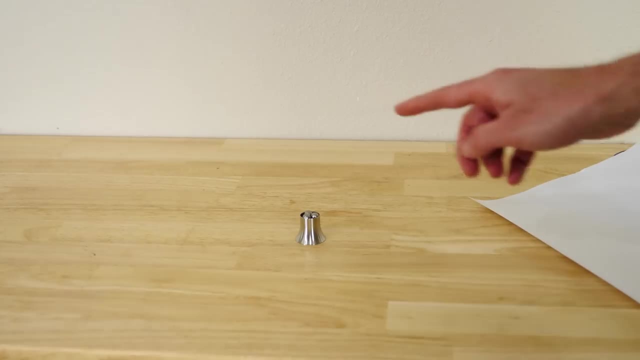 And then I'm going to just touch the tape and increase the resistance that way, So that will slow the spinning. But since it's flimsy tape it doesn't have a way to stop the precession. So let's see if I just press on the tape. 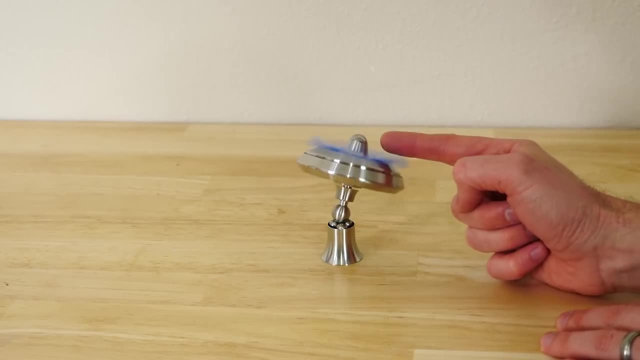 Let's see, if I just press on the tape while it's spinning, if it will actually cause it to rise up in the air. So that's pretty definitive: If you increase the friction of spinning, it causes it to rise up in the air. 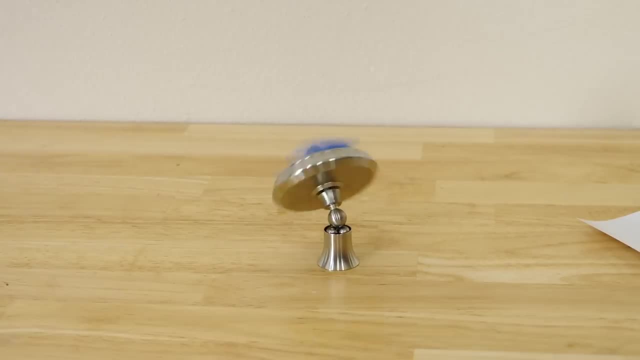 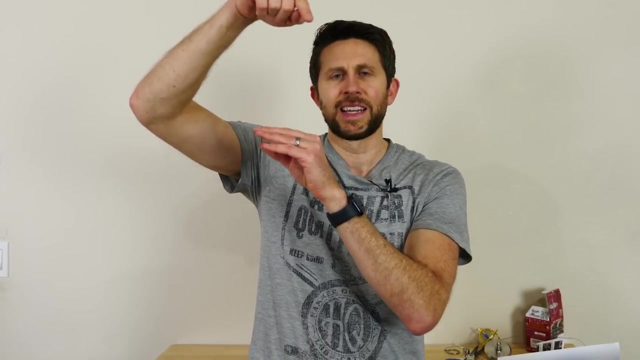 If you increase the friction of precession, it causes it to fall down. So it seems that there are two effects that can happen with a gyroscope: You drop it and it starts precessing. You drop it lower and lower and lower and eventually fall over. 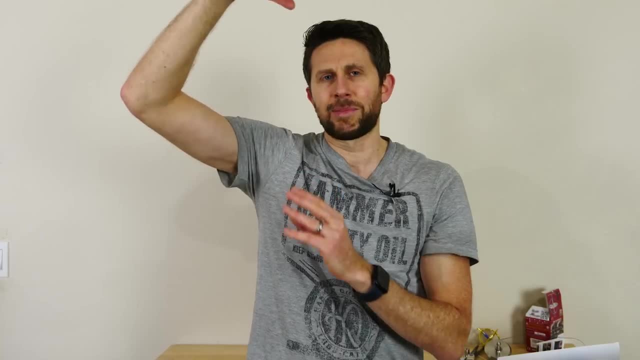 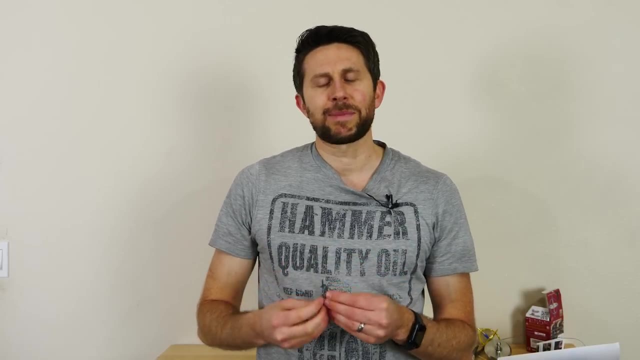 Or you let it go and it will get higher and higher and higher and eventually become stable at the top until it stops spinning and then falls over. So how does it decide what one it's going to do? Well, you have a balancing act between two frictions.